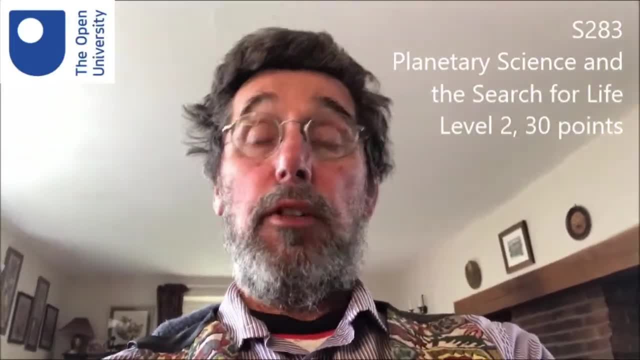 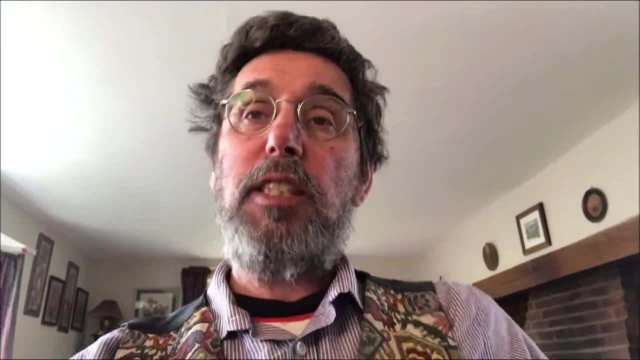 Hello, I'm Dave Rovery. I'm the chair of S283, which is Planetary Science and Research for Life. I've been asked to do a five minute introductory video and that's going to be a bit of a challenge, because I normally take half an hour or so. Okay, well, here I am. 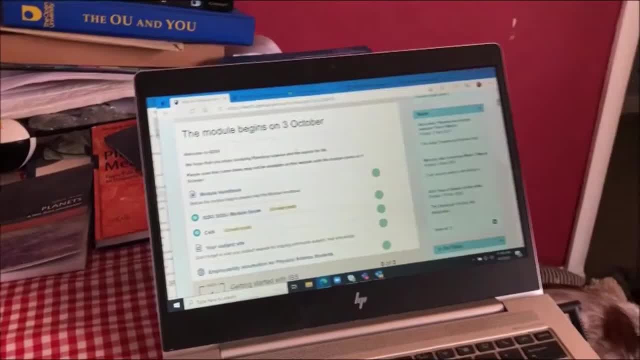 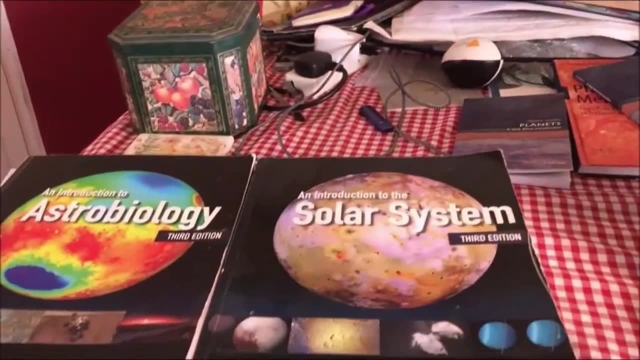 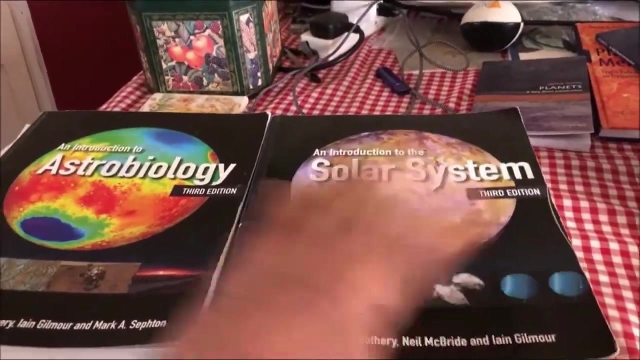 working from home. It's the second annual video I've done during lockdown. I've still got a, a dog at my side who is going to miss me when I start going back to the office. but this is where I'm working at the moment, and S283 is based around a couple of books which we wrote that 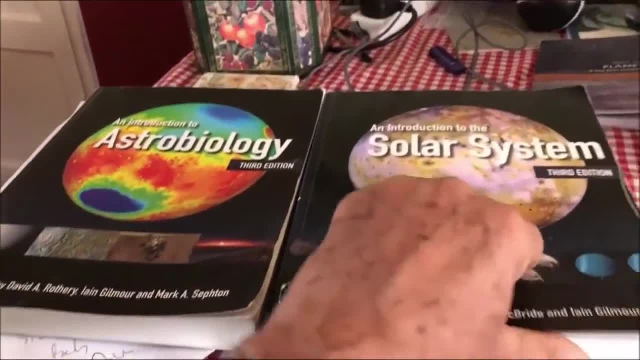 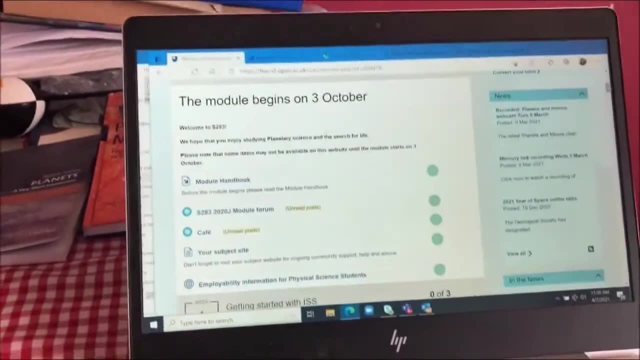 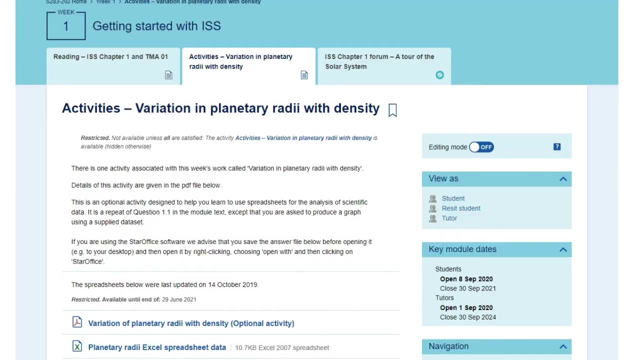 they're published by Cambridge University Press on the general market, but they're the basis of our course. This is where you get most of your content, but there is, of course, a module website and there are activities here and the various online things to do as well, and all your calendar is here online. 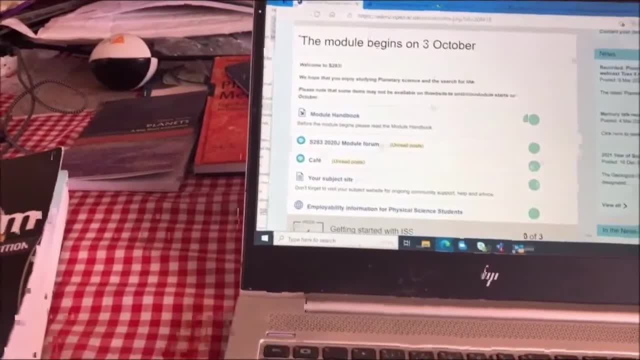 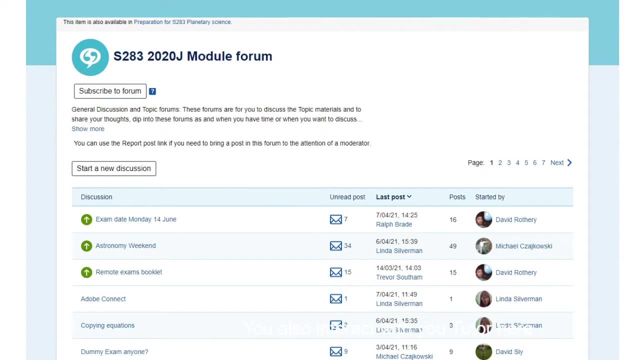 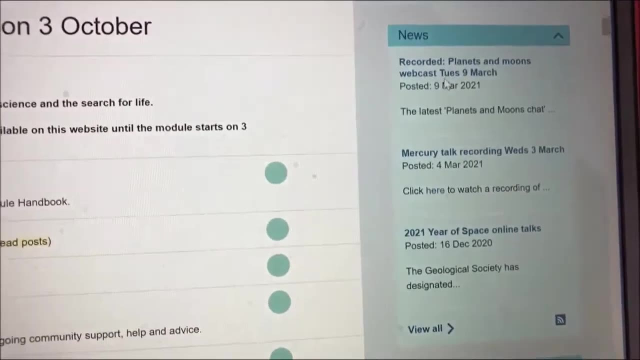 so this is where you will go to to see what's going on. There's a module forum and a cafe for more general chat, and there's a chapter by chapter set of forums as well, and there are news items about what's going on: our news that we've got this Planets and Moons webcast, for example, and also what's in the 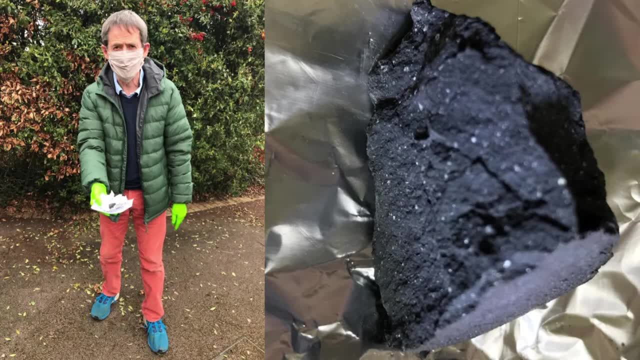 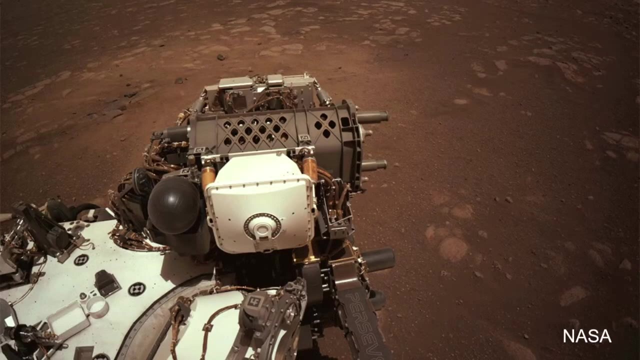 national news. One of the most recent news we've drawn attention to here is the Winchcombe meteorite, which fell only last week- It's about 40 miles west of where I live and the OU was involved in helping collect the fragments- and then the Mars Perseverance landing, which was in February. so we'll keep you up to date. 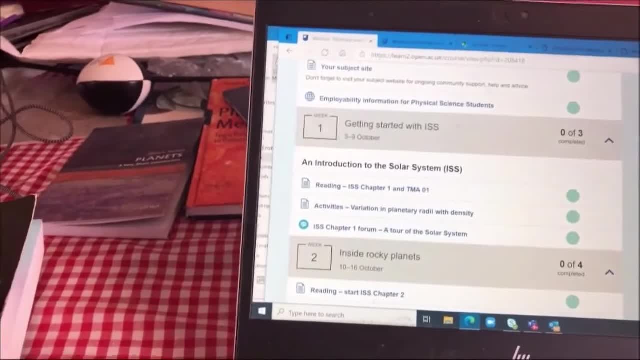 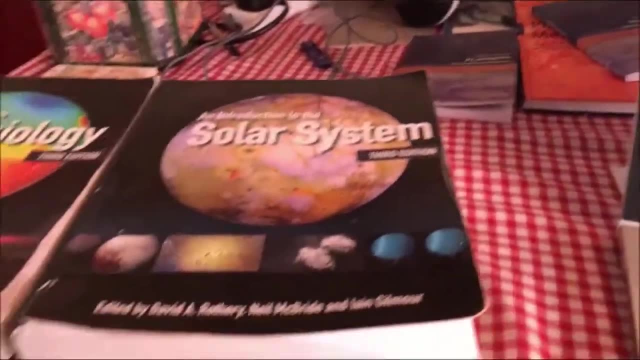 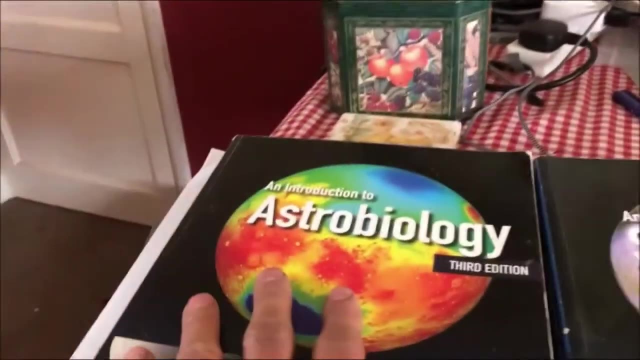 with news as well. I'm recording this in early April 2021 and this is really an introduction for students who are starting the module in October 2021.. So two course books. the first one is an introduction to the solar system, the second one is an introduction to 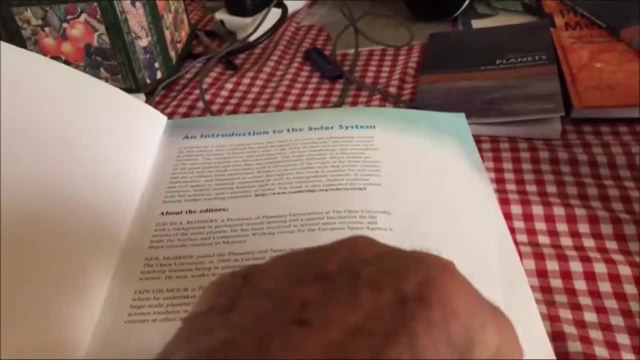 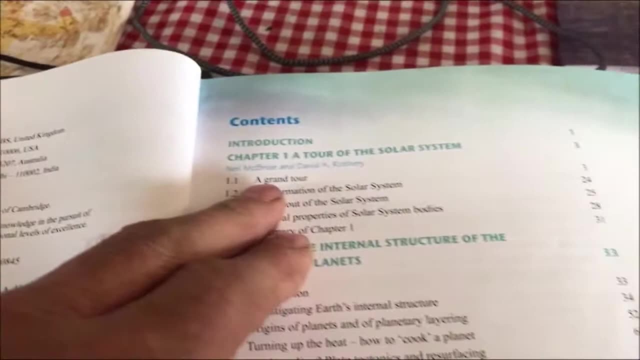 astrobiology and I'll just talk you through quickly what they cover. It's quite easy for me to show you the books rather than the screen. So we have an introduction to the solar system. give you a quick tour of the solar system to get your bearings. We're talking about the internal. 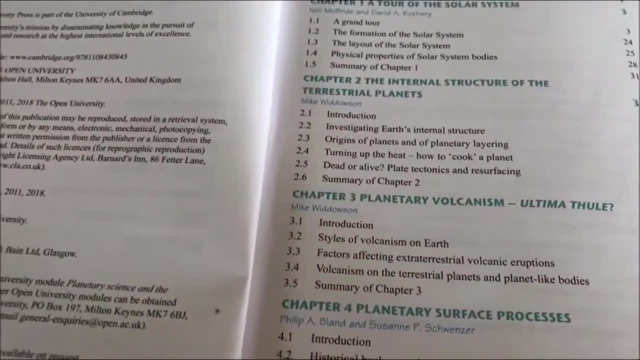 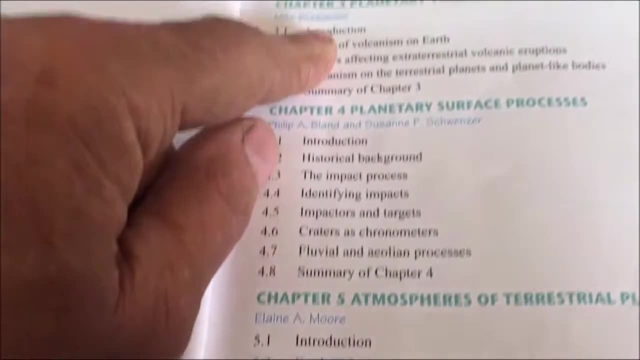 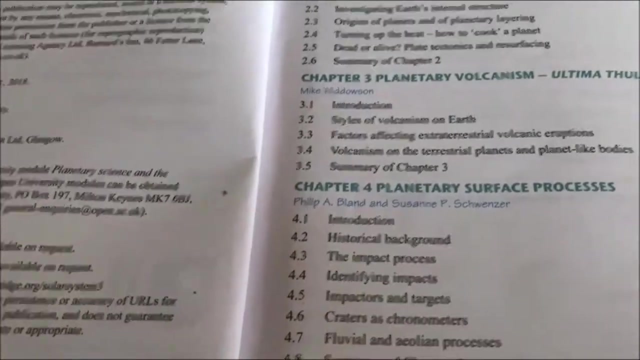 structure of terrestrial planets. Now, if you like geology or remember your geology from S111, a lot of this will be familiar. We talk about volcanism on planets and then we talk about planetary surface processes Largely cratering, because every planet with a solid surface has been cratered. but we talk about 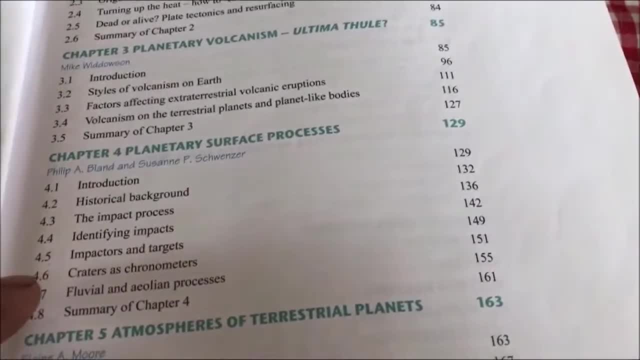 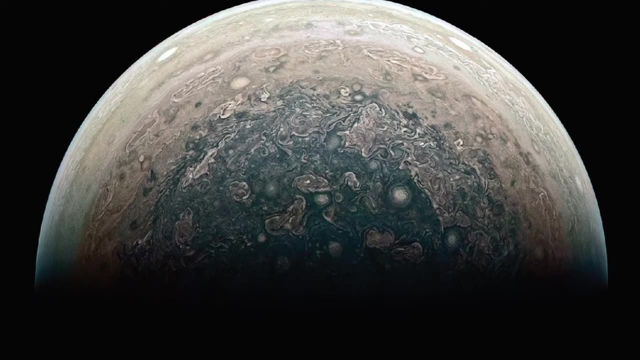 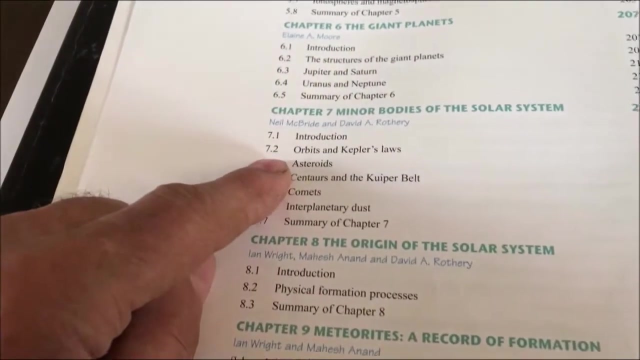 wind, blowing processes as well to an extent, and what rivers do. Then we look at the atmospheres of terrestrial planets. Then we go on to the giant planets- Jupiter, Saturn, Uranus, Neptune, Look at their interiors and their atmospheres. Then we look at minor bodies. 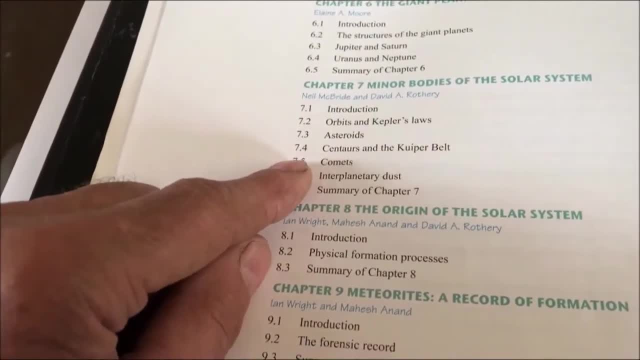 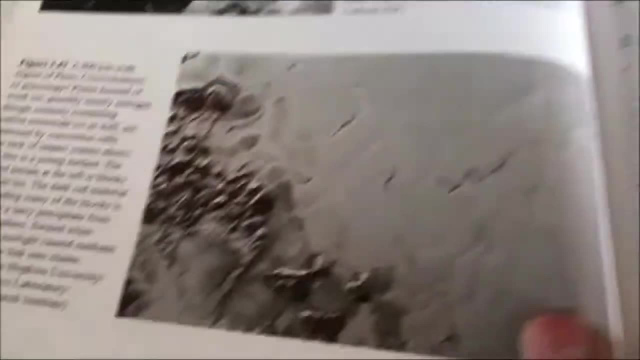 This is where we talk about how orbits work and we talk about asteroids and comets, Then the origin of the solar system and meteorites and what they can tell us. It's a richly illustrated book. I've happened on the chapter about planetary volcanism, So here's some icy. 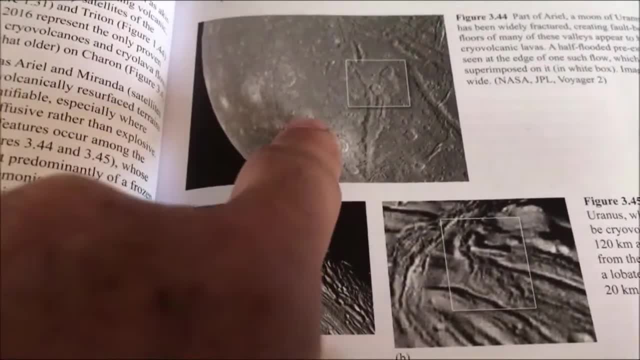 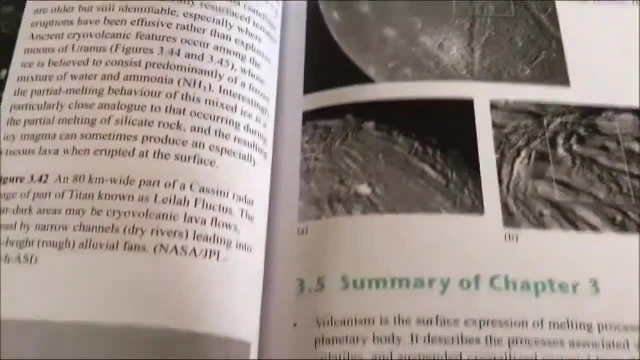 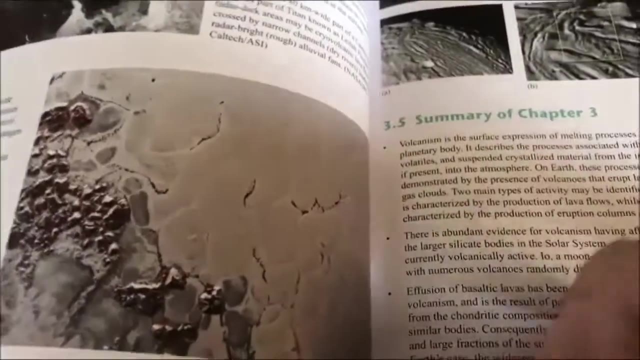 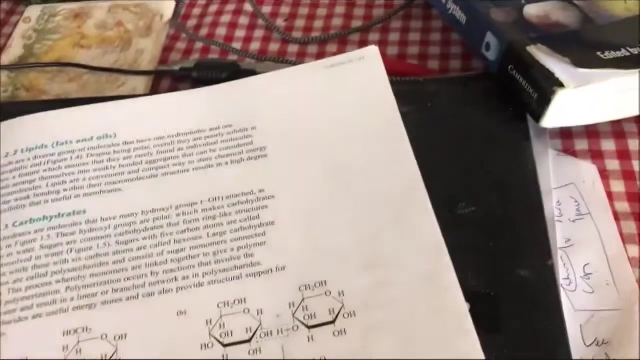 volcanism spilling out of canyons on Ariel, a moon of Uranus, and here's an icy flow on Miranda, another moon of Uranus. Here's weird icy convection patterns in nitrogen ice on Pluto. Moving on because they've given me five minutes. Introduction to Astrobiology begins with talking a. 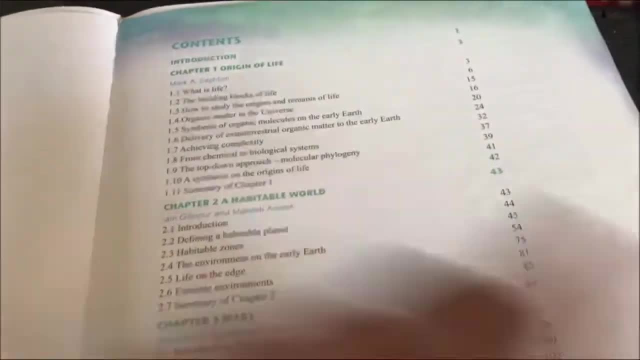 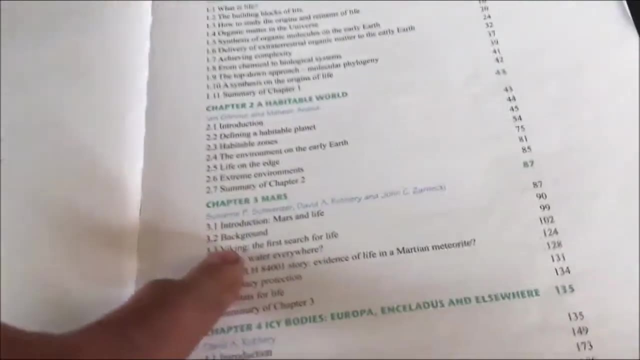 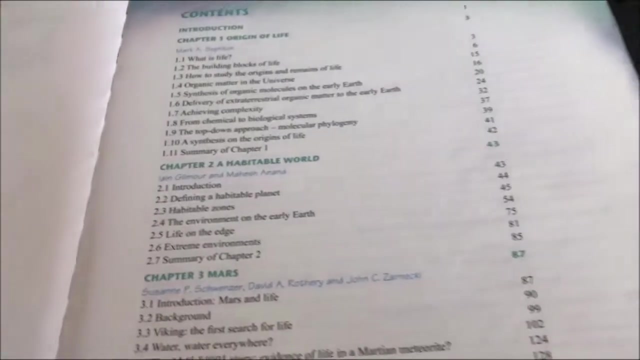 little bit about life and how we recognise life, how it might start, what it takes for the world to be habitable. Then we look at Mars in the context of when it might have been habitable. Then we're talking about planetary habitability. We're really talking about microbes here. 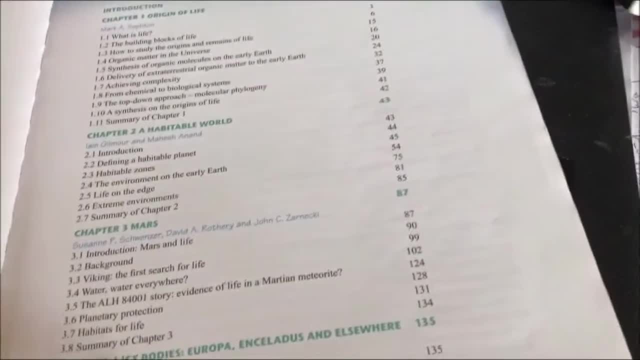 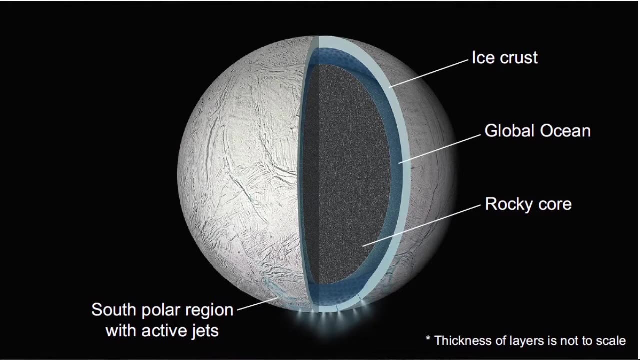 not complex organisms. We look at icy bodies Now. inside some of the icy moons, Jupiter and Saturn, there are internal oceans. We're very sure of that now. But whether there are habitable niches inside those oceans where life could exist, powered by chemical energy? 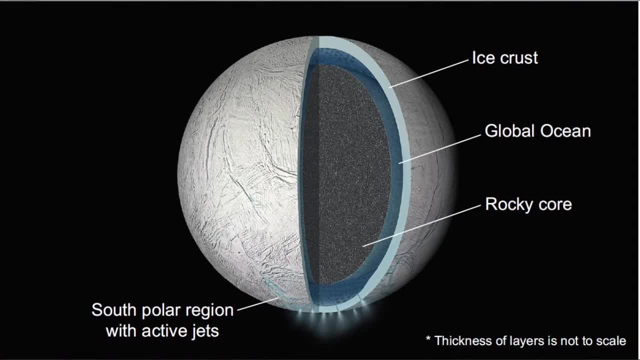 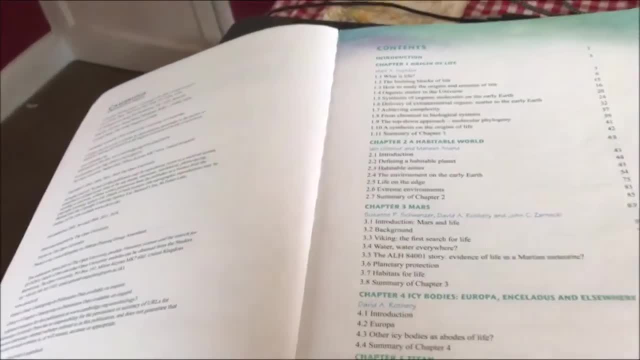 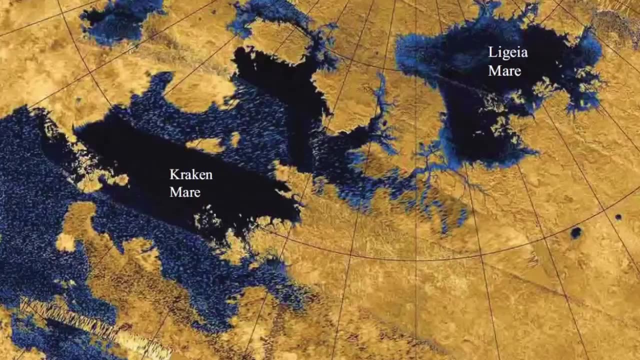 we're not sure, But it's quite likely. you could take organisms from Earth inside Europa, put them on the floor of its ocean and they would survive. It's whether life has started there in the first place, but it's the big unknown Titan, the moon of Saturn, with a marvellous atmosphere.